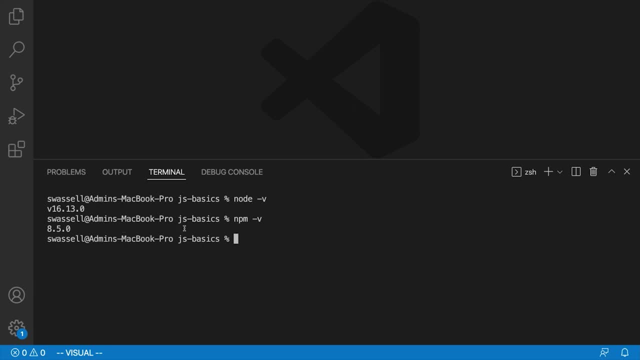 a version for that as well. If you just see something like command not found, then that means you don't have it installed And you'll need to do the instructions I'm about to show you. So, assuming that you don't have Node and NPM installed, what you're going to want to do is go. 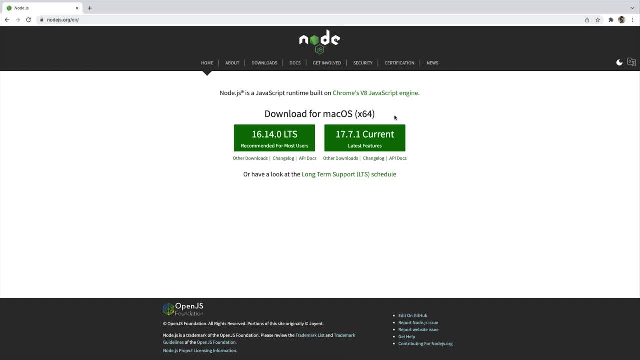 to nodejsorg And you're going to want to download it Now on this page. there are two main options that you have for downloading Nodejs. One is the long-term support version and the other is what's called the current version. Now, for most people, as Nodejs' website itself says, the long-term 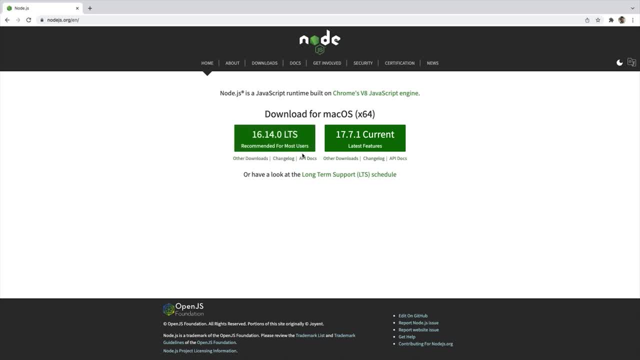 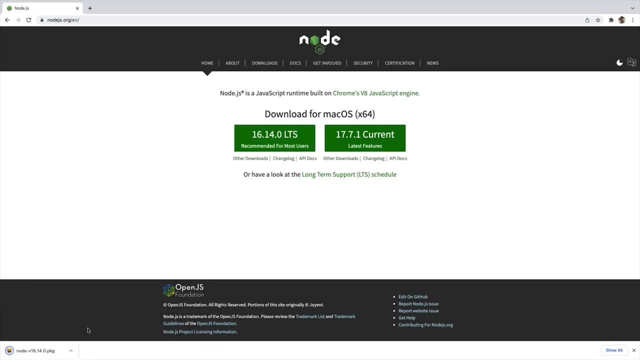 support version is going to be what's recommended. It says recommended for most users. So what I'm going to recommend you do is click on this button, which will download the package for installing Nodejs, And once that's completed, you're going to want to click on that and it will. 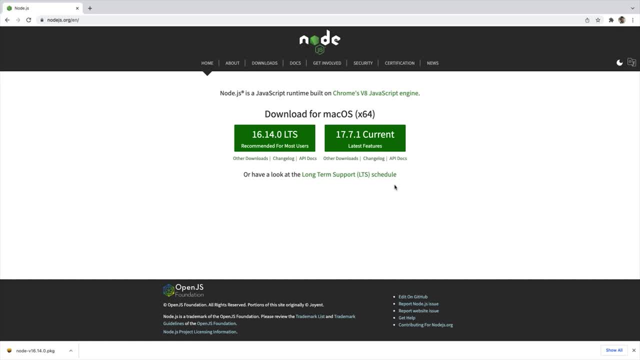 walk you through the installer wizard Now if you are feeling more adventurous. I wouldn't recommend this right now, But if you ever want to work with the latest features of Nodejs, all you would need to do is just come in here and select the current version instead, And again, you're probably going. 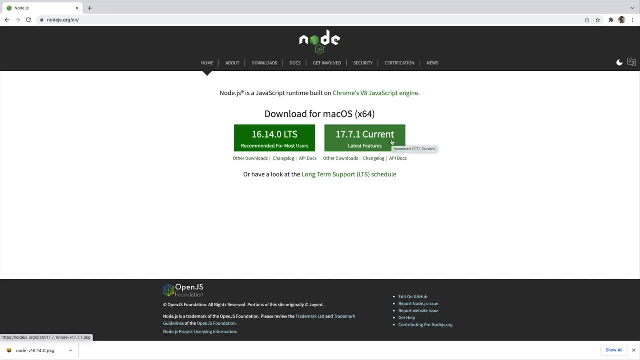 to be seeing different versions of this than I am right now, because, chances are, versions will have advanced quite a bit since I recorded this, But everything that I'm about to show you is going to still work exactly the same way. All right, so let's click on the installer that we just downloaded. 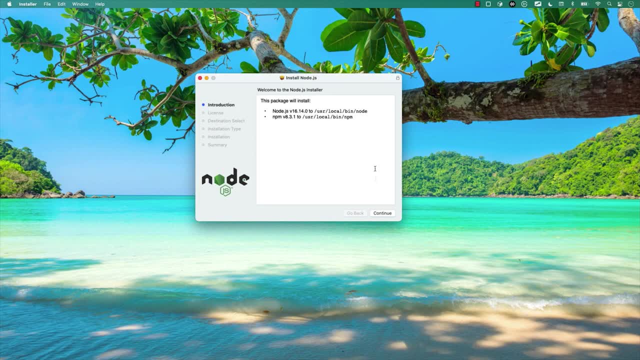 And what that's going to do is open up the installer wizard. We're just going to click on continue, continue, agree and install, And what that will do is it'll probably ask you for your password, So I'm going to enter mine there, And then what we're going to see is it'll just install. 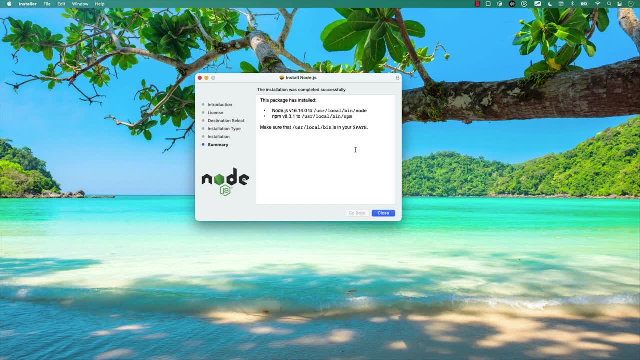 everything. for us, It usually takes, you know, a few seconds max, And then, of course, depending on the system, you're going to want to follow the directions that it displays here. I've already done that myself, so I'm not going to do that again And we're just going to click on close. 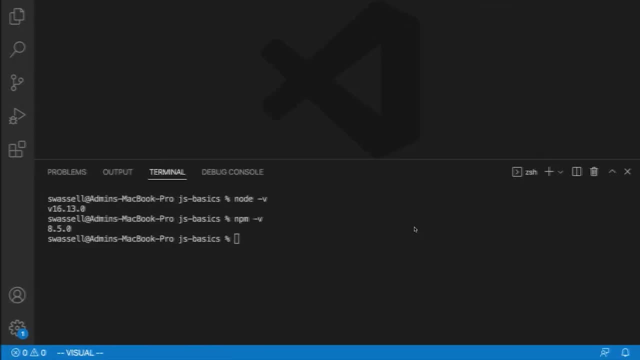 All right. so now that we've installed Nodejs, we should be able to go back to our terminal here, and we may want to close it and reopen it. just to restart the terminal. Oops, it looks like we need to click on the trash can button instead, And then we'll open up a new one here And now. 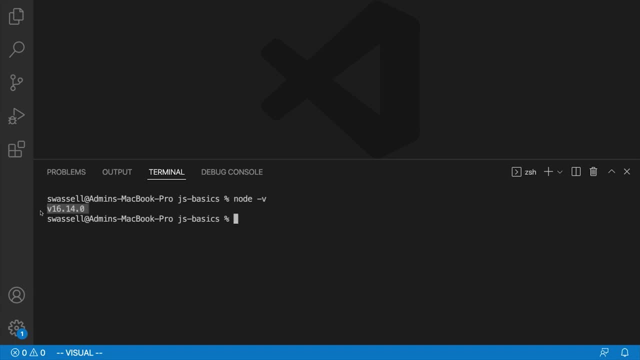 what should happen is, if we run node-v, we should see that we have a new one, And if we run node-v, the latest version that we saw inside here- right, the long-term support version that is displayed there. And if you run npm-v, you may see a different version there as well. 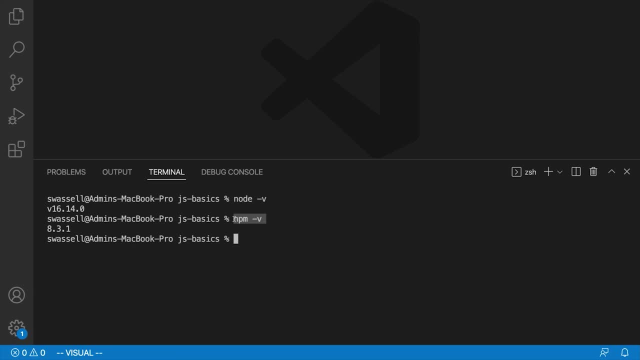 Now npm is actually bundled with Node, So by installing Node, as we just did, you're going to have access to npm as well. right, You don't need to install that as a separate thing. Okay, so now that we've installed Nodejs and npm locally, I'm going to show you how to run backend JavaScript. 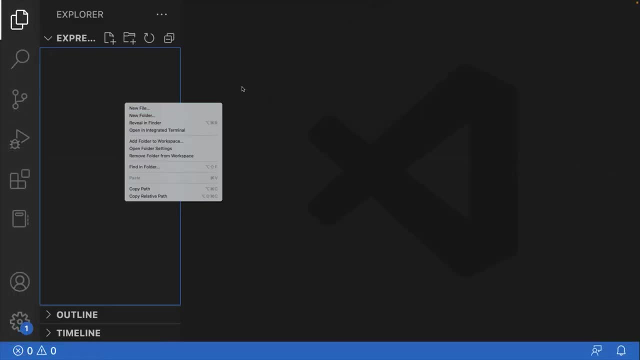 code using Nodejs And I'm going to show you how to run backend JavaScript code using Nodejs. What we're going to do here is we're going to start off by just creating a new Express application. It's going to be a very simple project. So actually I'm just inside this. 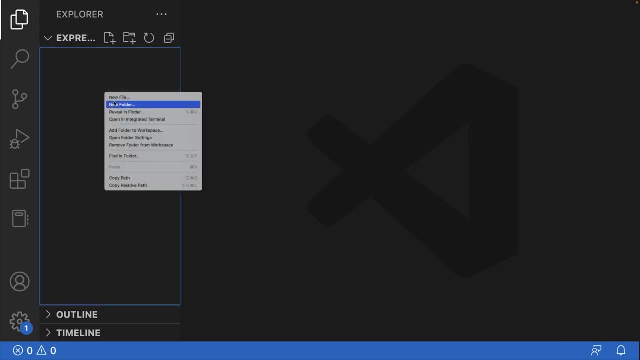 folder called Express Course, And inside here I'm going to create a new folder which I'll open up in my IDE And we'll just call this new folder something like front-end-basics. And I'm just going to open this up in my terminal by saying code and then front-end-basics, And that'll open. 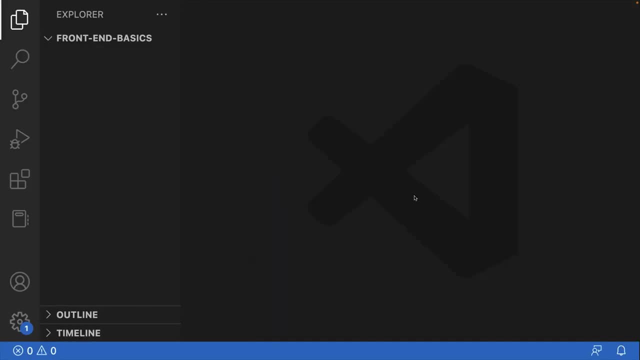 that up in another IDE window, Cool. So first things first, let's just initialize this as a new npm package by saying npm init, dash y. That'll create the packagejson file for us, And then we're going to go and install express by: 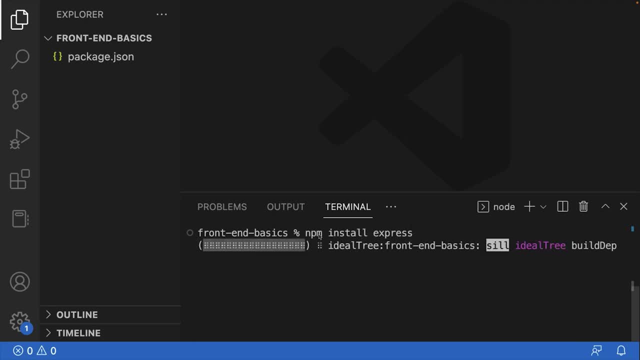 saying npm, install express, And once we've done that we can create our new server by just creating a new file. And actually I'll create a new folder called source And inside here I'll create a new file called serverjs, And then we're just going to set up a very simple 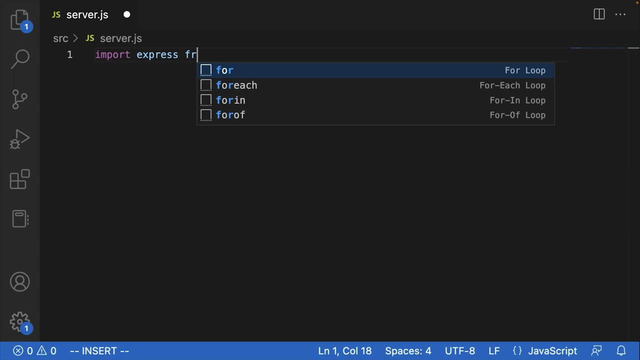 express server by saying import express from express And then we'll say const app equals express. There we go. And then we'll tell our app to start listening by saying applisten, And we're going to have it listen on port 8080.. And then inside this callback here, just like we've 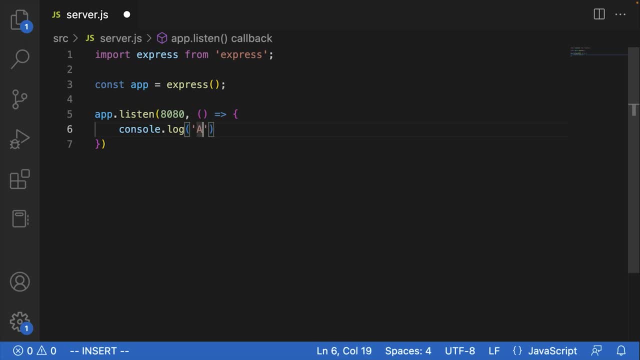 done previously. we'll say consolelog server is listening On port 8080. So none of that should be new to you. I'm sure you could do that, probably with your eyes closed at this point, But nevertheless we now have a handy express server that we can use. 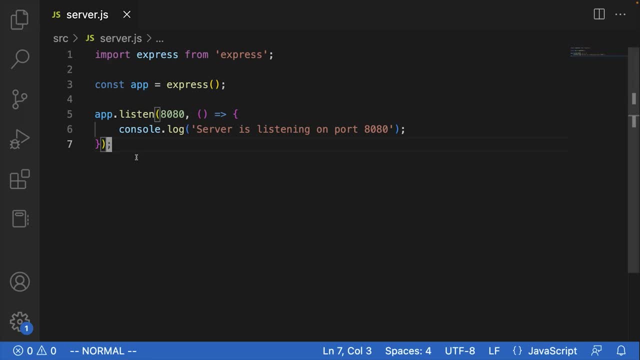 for demonstration purposes, All right. So the next thing that we're going to do here is create a file that we're going to send back to the front end when the front end sends a request to our server. And this is the first step, really, in starting to execute some of our code on the 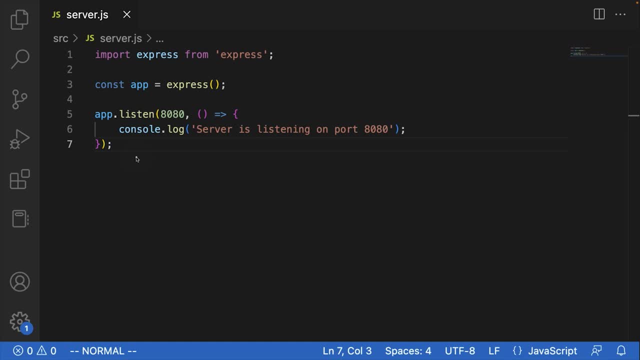 front end is we're going to need to send the front end a file containing some of our code. It's going to be some sort of code that we want it to execute. So what this is going to look like in our first example here is when our server receives a request from the client. 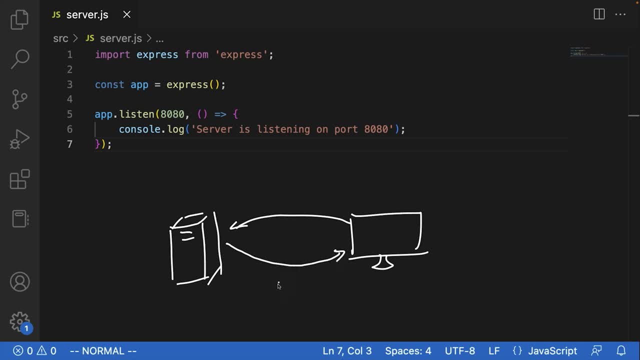 the server is going to send back a file- And this is going to be an HTML file, by the way- containing some scripts inside of it. We'll talk a little bit more about how that works in a minute. And when the client receives this file, what it's going to do is it's going to render all of the 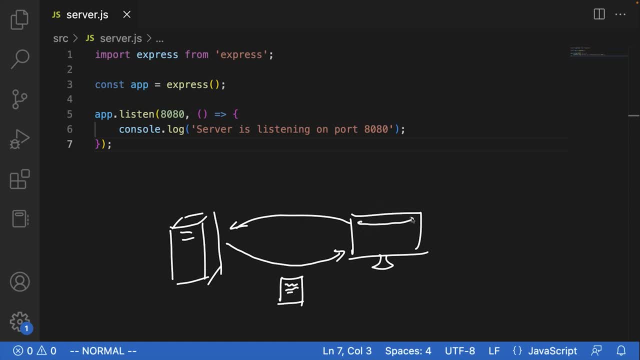 JavaScript code. And, by the way, we're going to be sending this request using a browser on the client side instead of something like Postman- although it's perfectly possible to use Postman for this testing as well- But so when the browser receives this file from our server, what it's? 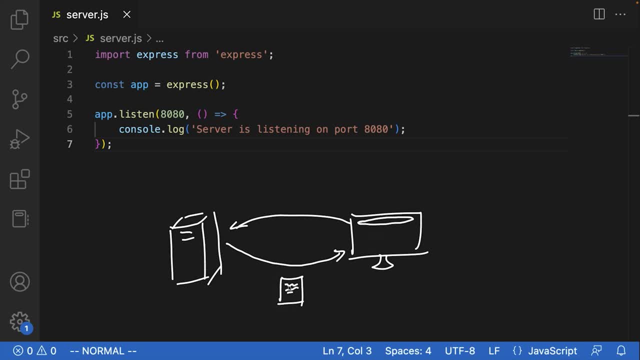 going to do, as I said, is go through and render the HTML, And somewhere in that HTML we're going to add a script tag with some JavaScript code inside of it. right, So we'll be able to execute front end JavaScript code. And what the browser is going to do is it's going to send a file to the 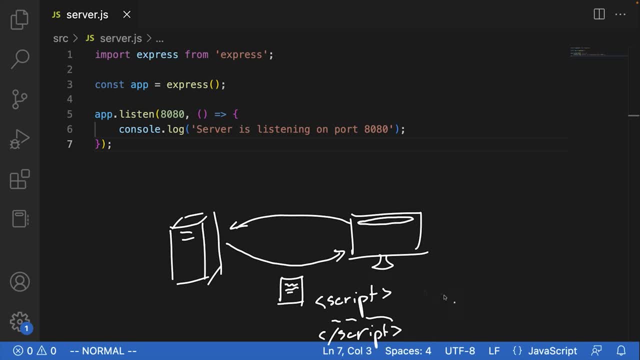 client side And what the browser is going to do when it reaches that script tag is it's going to automatically execute the code that that script contains. So this is how we are really able to start defining what we want the browser to execute from. on the back end is we can just choose what. 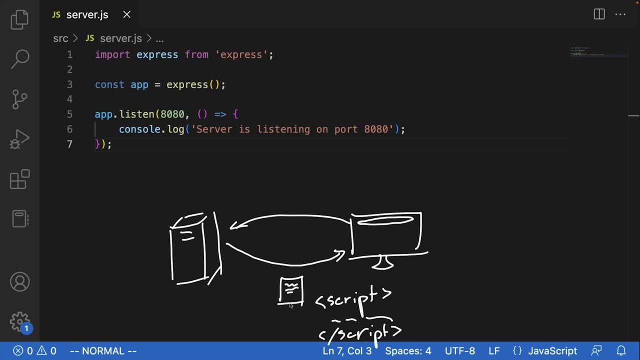 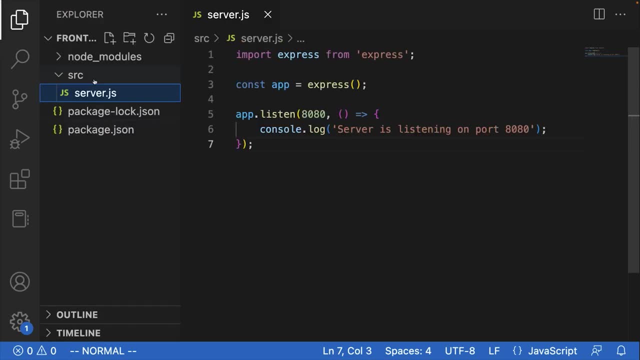 sort of JavaScript code we want to put in this file we're sending back. Okay, So in order to do this, what we're going to do is just create a simple HTML file, And you can create that just inside this source directory as well. 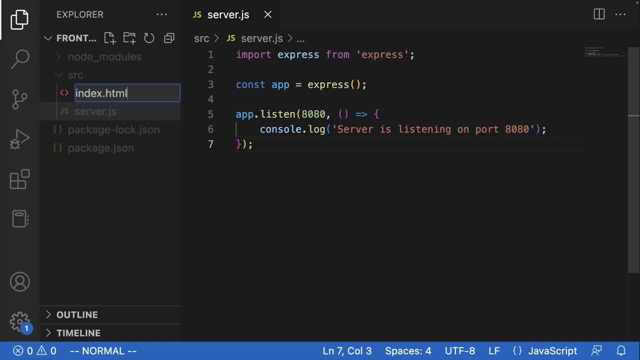 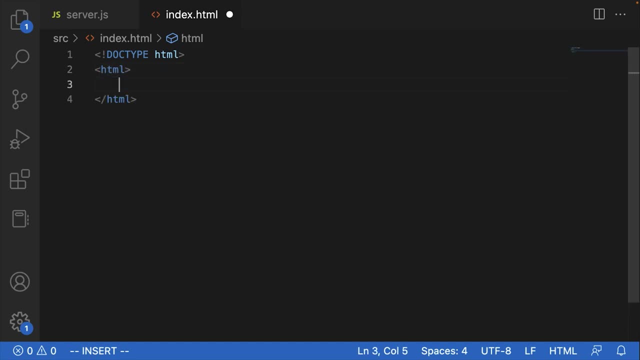 So we'll say new file, And then we'll say we'll just call it indexhtml, I suppose. And let's just set up a very simple HTML file here. we're going to have the doc type HTML. then inside the HTML 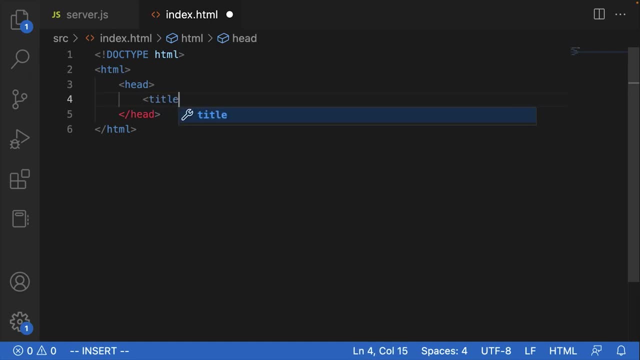 tags. we'll have the head And let's just add a title to this page. we'll say something like front end execution test. And then for the body, we're just going to have a simple H1 heading that says something like this is a test, right? That's not going to be a test, right? That's not going to. 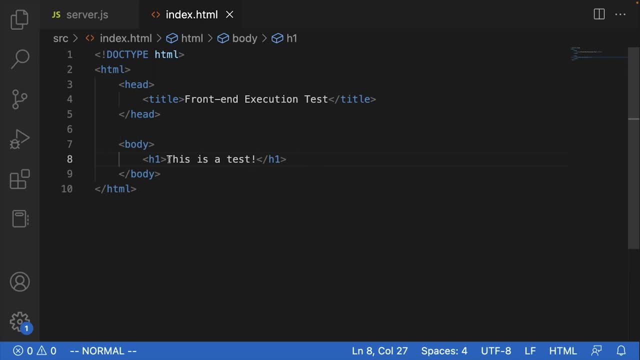 be a test. That's not really necessary, but it just gives us something to display in the browser so that we can see we've actually received the file. And underneath this- and really this could be anywhere in the HTML document. we'll discuss that in a little bit more detail later on. Underneath: 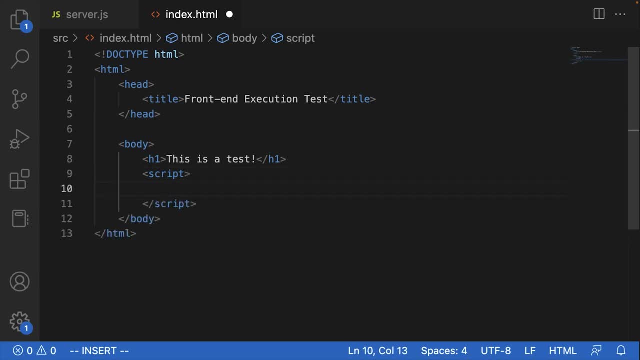 this: we're going to put a script And in between those script tags, as I said, we can start writing JavaScript code. So the simplest piece of code that's really only available in front end JavaScript, for the most part, is going to be a function called script, And then we're going to have a function. 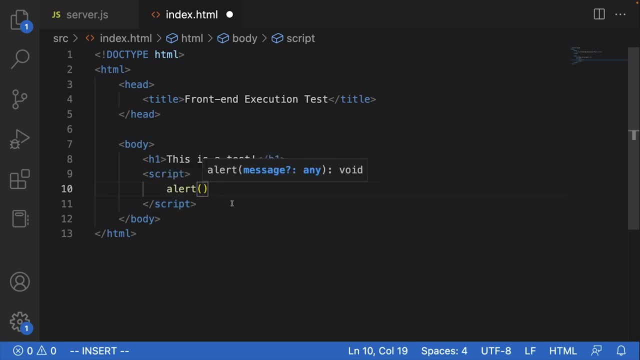 called alert, which will just display a little pop-up window in the browser. You'll see what that looks like in a minute, But what we're going to do is have that alert say something like hello from the front end. Okay, So that's our simple indexhtml file. So now what we're going to need. 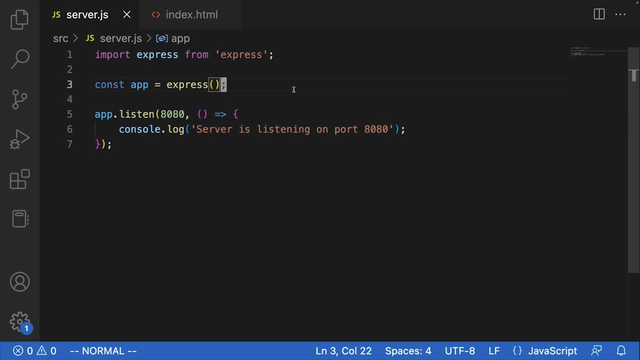 to do is have our server send that file back to the front end as a response when it receives a request. So what we're going to do is just define a simple get endpoint That will listen on the home route And then inside the callback here we're going to have the request. 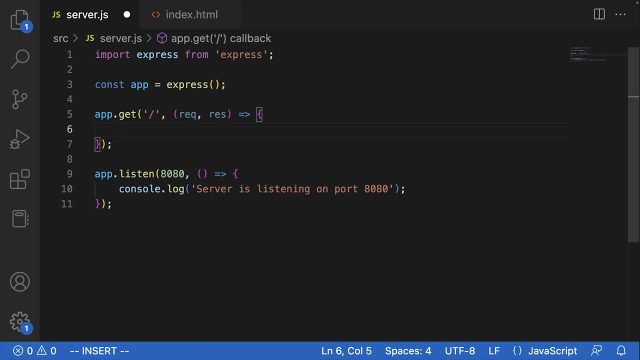 and response, of course, And in order to send back a response with that HTML file in it, what we're going to do is say responsesendfile. So this is the function that we're going to use to send back files specifically to the front end right, Instead of doing something like responsejson when we 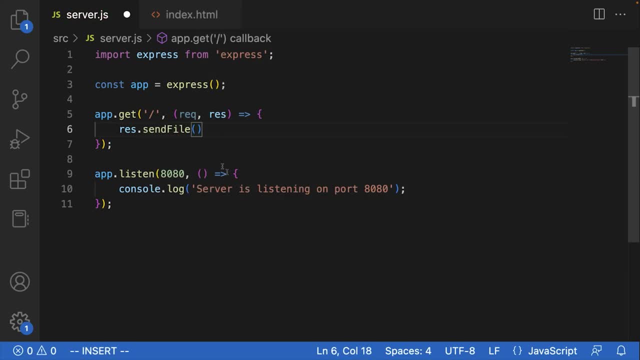 wanted to send back JSON data, So responsesendfile, And then we just need to provide the path to the file we want to send back, which is of course, going to be. actually. we'll import the path library here, So we'll say: import path from path. 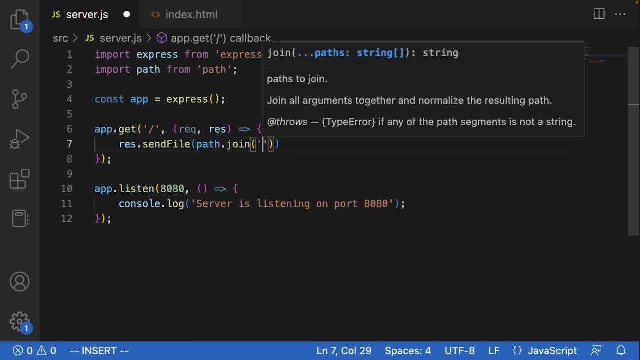 And then down here we're going to say pathjoin, And inside here we'll say underscore, underscore, directory name, And this is just going to be indexhtml. Okay, So now that we've done that, we should be able to load this indexhtml file by sending a request to our server from. 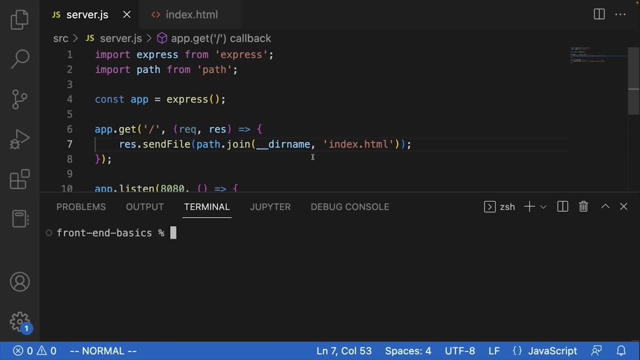 our server. So we're going to do that, And then inside here we'll say underscore, underscore, our browser. So what we're going to do is start up our server by just saying node serverjs, And oops, that should actually be source slash serverjs. There we go, And oops, it looks like. 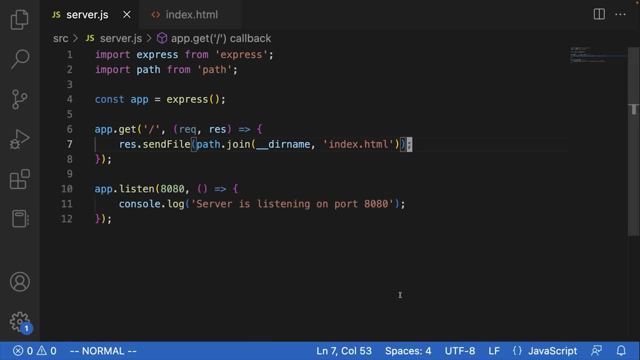 we got another error because of the import statements And actually in order to avoid having to do all the funny stuff with this directory name thing here when we convert our project to module, I'm just going to switch these things up here to require statements. So 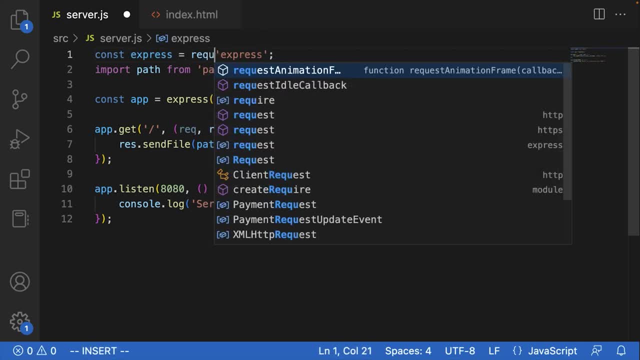 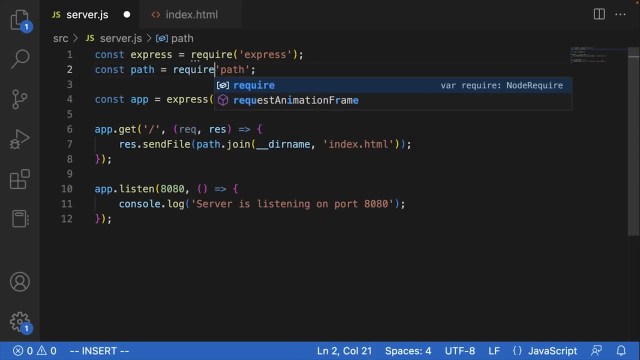 we'll say const express. And same thing with path. We'll just say const path. equals require path. Okay, So let's try this again. We're just going to run our code one more time And sure enough, we see, server is listening. 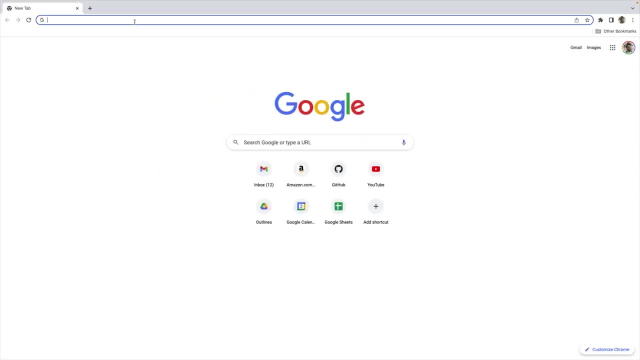 on port 8080.. And if we go over to our browser now and go to localhost 8080, sure enough, we'll see that our code is executed and we get this little pop-up window which is an alert that says hello from the front end, Okay, And if we click okay, we'll see that everything else. 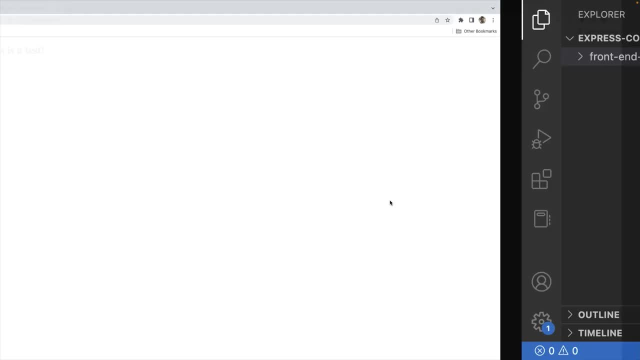 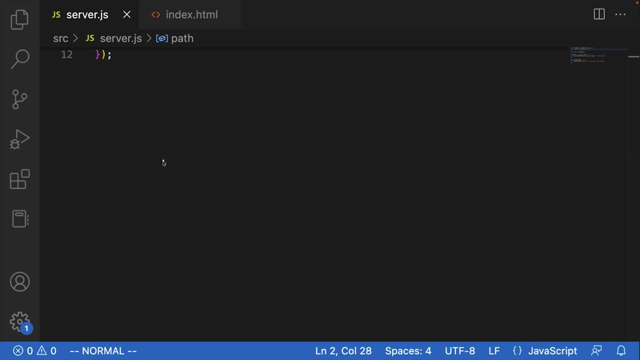 will be rendered in the browser. So again, what's happened here is our browser. I'm just going to draw this out one last time here to make sure we have the visuals to go along with it. What's happening is we have our server running over here and our browser over here sends a request to the. 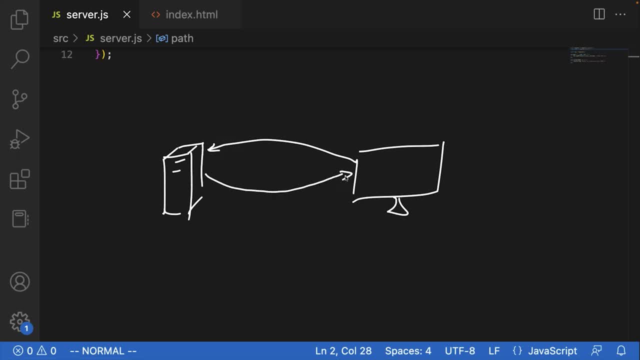 server. The server sends back that indexhtml file to the browser And then our browser basically goes through that file, You know, parses all of the HTML And when it reaches that script it executes the script And that's where we see the little alert displayed. Okay, So we were successfully able to. 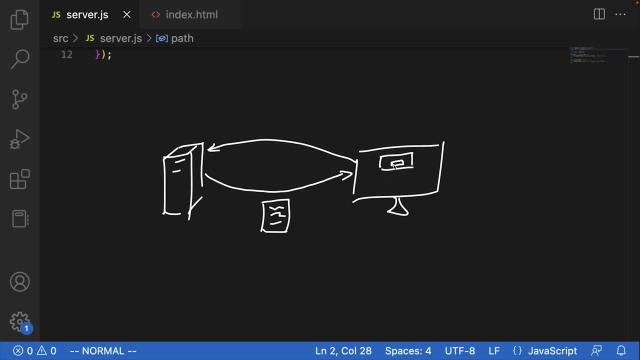 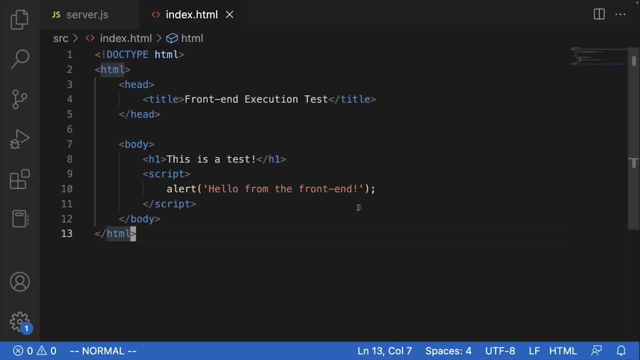 run a little bit of JavaScript code in the browser now, which is our first piece of front end executions. All right, So if you want to play around with this a little bit, what you can do is just change some of the code that's in this alert. If you want to right, you can write the. 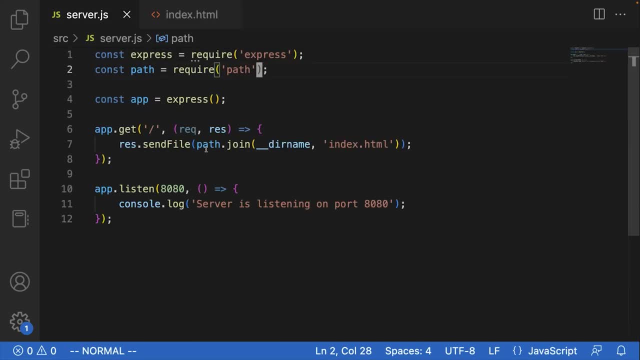 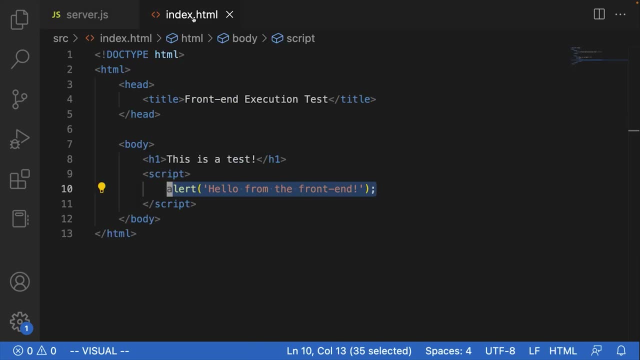 same kind of JavaScript. for the most part You can write on the back end. There are obviously some things you can't do, Like you can't access the file system like you can on the back end, because well, obviously the browser isn't. 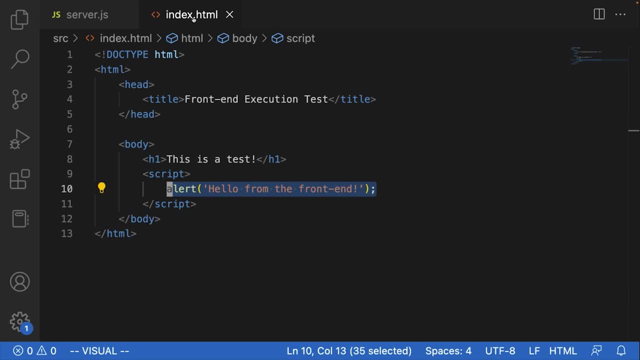 going to let you access your user's file systems on the computer. they're visiting your site on, You know. but if you wanted to do something, for example, like log something out to the console, right, Consolelog works on the front end, just like on the back end. But what it's actually? 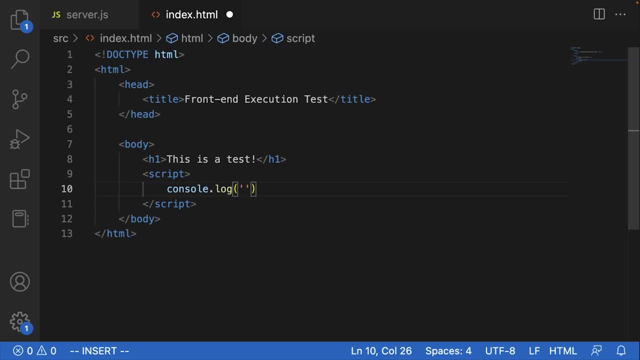 going to do is print that out to a slightly different place, Just to show you what this looks like. we're going to say consolelog And again we'll say hello from the front end And if we head back to our browser now and hit refresh, what this is. 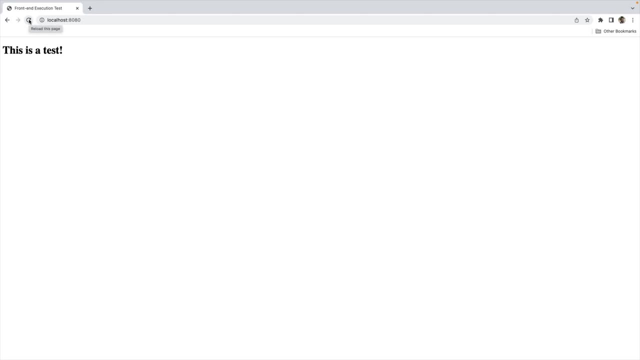 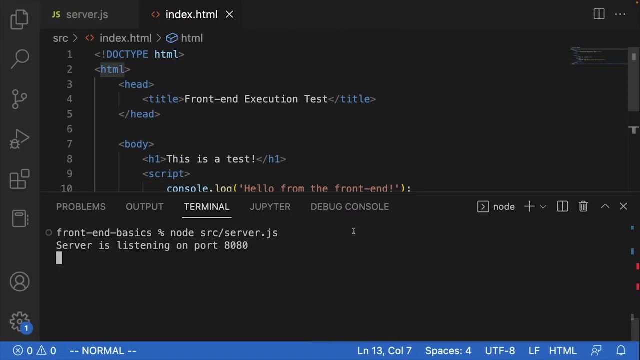 going to do is send another request to the server and load that updated indexhtml file with the changes we just created And actually, as a matter of fact, we need to restart our server. So what we're going to do, actually, in order to avoid having to restart our server every time we make. 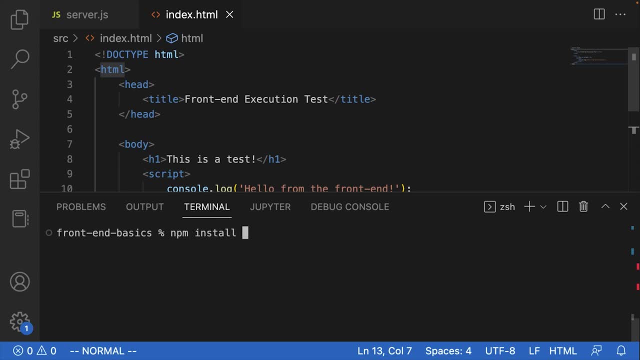 a change. we're just going to say OK, so we're installing the Node Demon package and we're going to use that to run our server continuously. So once that installs here, just give that a moment And then we can run our. 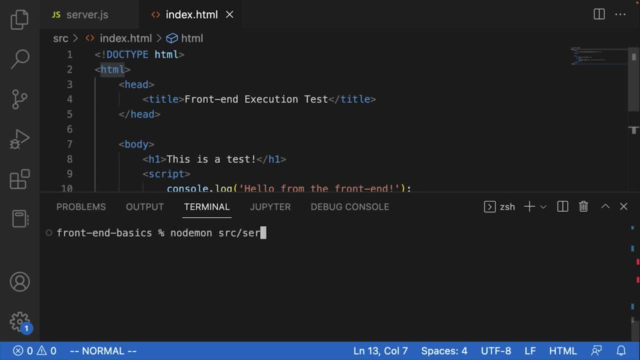 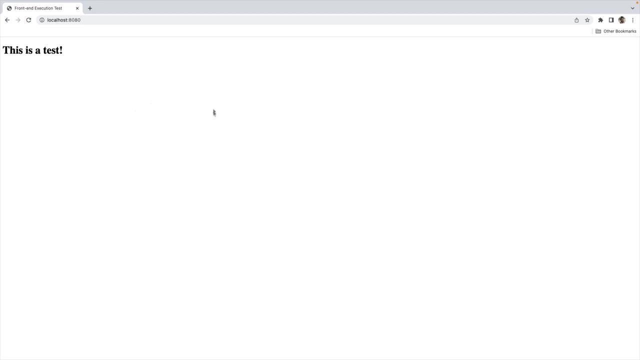 application by saying Node Demon and source slash server dot js. Oops, and that should be: npx. Node Demon, source slash server dot js. OK, so now that we have our server running, we should be able to go back to our browser and hit refresh, And what we see here now is the new indexhtml file that we received. 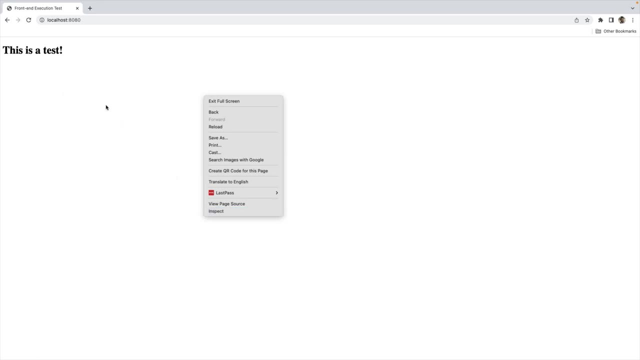 That's not really obvious because there was no change here, but we know that because the alert wasn't displayed again. So if you want to see what we logged out to the console on the front end, what you can do is right click and then click on inspect. And if you go to the console, 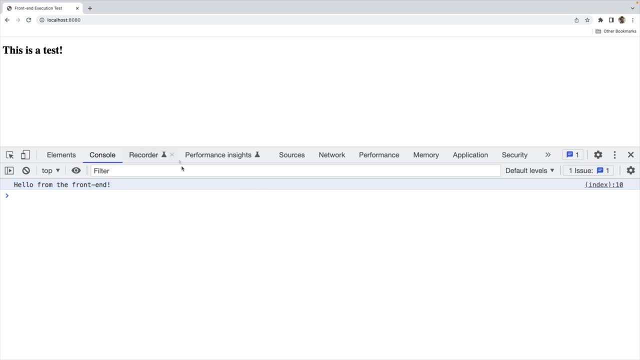 sure enough, you'll see the message there that says hello from the front end. So this is the front end console right? This is where things will be logged out when you say console dot log on the front end And on the back end, obviously, if you log something out. 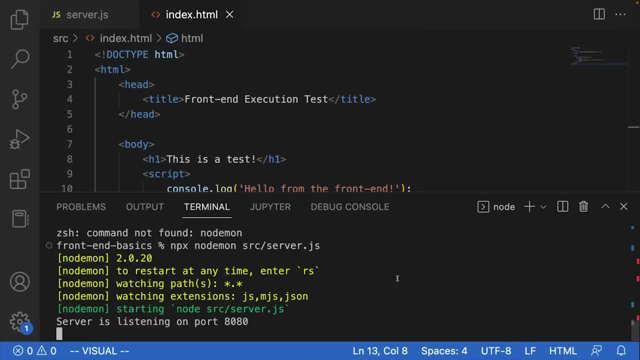 you're going to see that in the terminal, All right. So anyway, what we've seen here is the basics of executing code on the front end, when we wrote the code as part of an express application. So far, it might not be apparent to you what sorts of things we might actually. 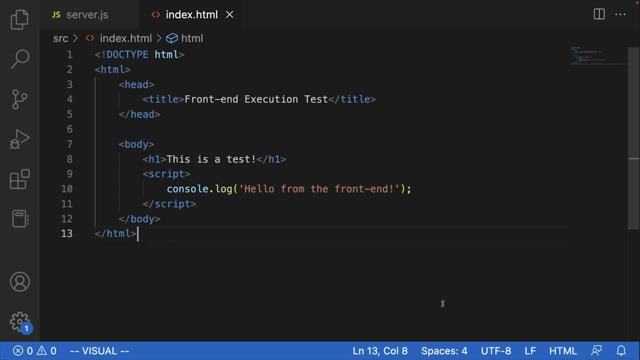 want to do on the front end, right? In other words, what are some things that we could do on the front end that would actually be helpful to our app as a whole, instead of just, you know, doing things like displaying an alert or logging to the console? Well, that's what we're going to. 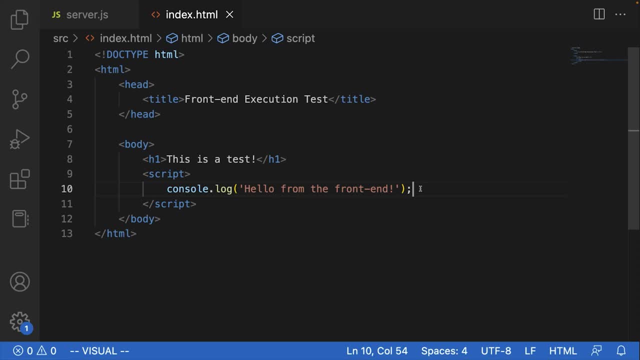 take a look at here, And one of the first things we're going to take a look at is, in my opinion, one of the most effective things that front end code can do. What we're going to take a look at is how to have our front end code load data from our back end code, So, in other words, the logic. 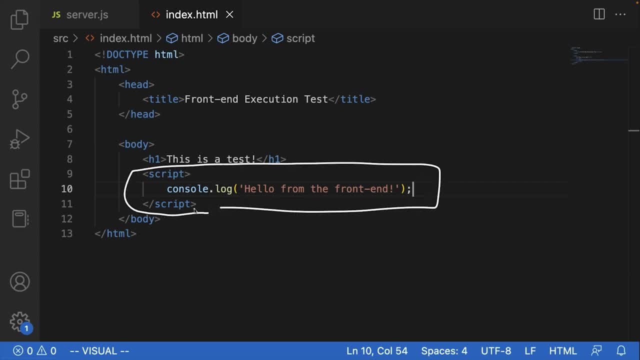 that we put inside these script tags here many times is going to want to have access to some sort of application data, And so what we're going to do is we're going to take a look at if we were creating some sort of e-commerce site that displayed all of the products, all of their. 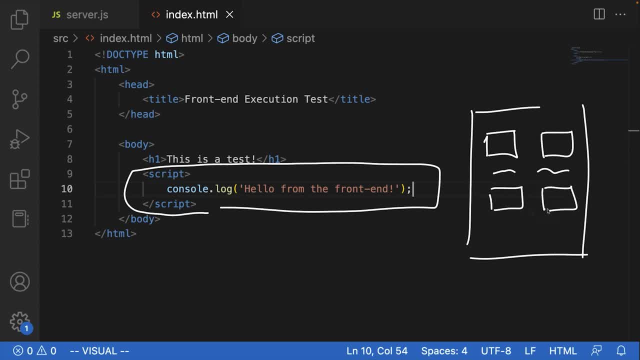 prices, et cetera, right, I'm just going to draw those like this. Then, obviously, we're going to want our front end to be able to load all of that product data so that it can display it in the interface here, right? And we're also going to want the front end to be able to do things like 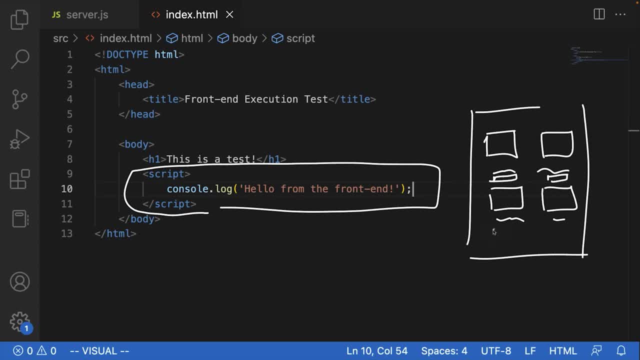 add items to cart when the user clicks the button for an item, and you know other things like that. So, in other words, there are lots of situations where the front end is going to need access to the same sort of data that the back end usually. 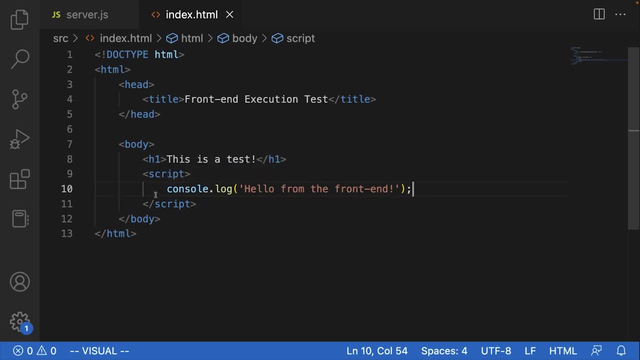 gets to work with, And in order to do this, we're going to have to actually write some code inside our front end scripts that will itself make a request to the back end. So this might sound a little bit confusing. Let me just draw this out again. I'm going to be drawing the same. 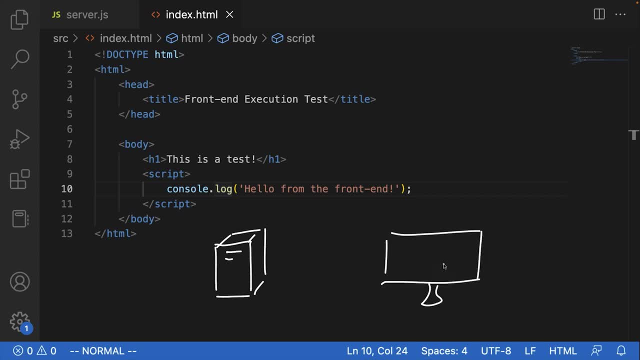 server and computer, probably about a hundred times during this course. All right, but just to try and make things extra clear for you, when the client first requests the front end, they're going to have to send a file from the back end, right, The back end is going to send back that indexhtml file. 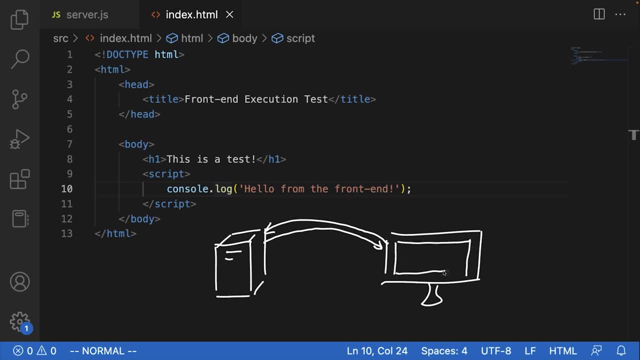 and the browser is going to render that file inside itself so that we can see things like the interface, And it's also going to run any scripts that it finds in the HTML. All right now, what we're going to do here is actually have the script itself, which is, hopefully you can see. 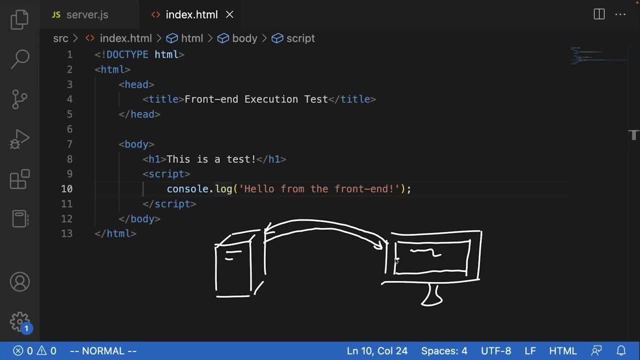 it represented by this inner box. here We're going to have the script itself make a request to the server, and the server is going to send back some sort of JSON data that our front end will then be able to use. All right, so in other words, there's two things going on here. The first thing 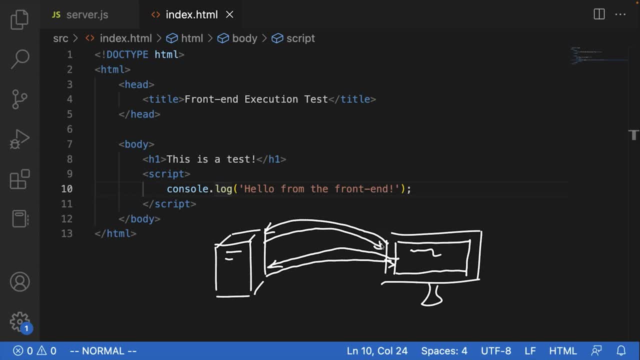 is the browser loading the initial file from our server right When we type localhost 8080 into our browser and hit enter, All right. and then the second thing is when our browser actually runs the front end code that we wrote inside this script tag, and that code makes a specific request. 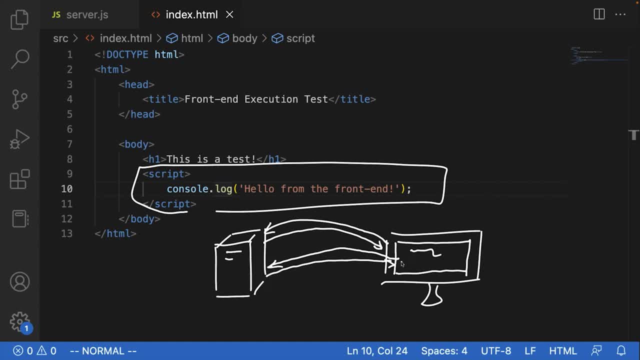 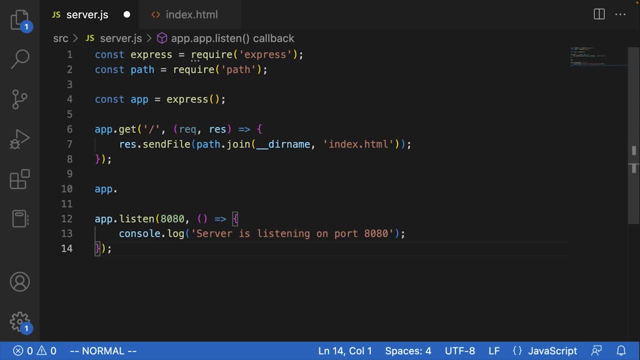 to the server and gets a response back. So hopefully that's making sense so far. In order to make this work, what we're going to do is open up our serverjs file and we're going to create a separate endpoint that our front end code will be able to load data from. So this endpoint up here. 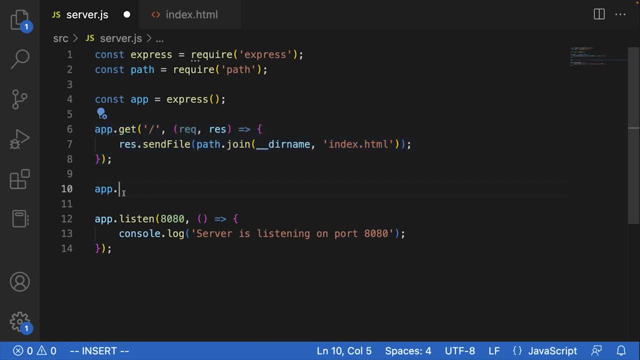 was meant to allow the front end to load a file. The one down here is going to send back some data. So what we're going to do is we're going to say appget, and for the path here, we're actually going to say get slash API, slash users, And what this is going to do is it's simply going to return. 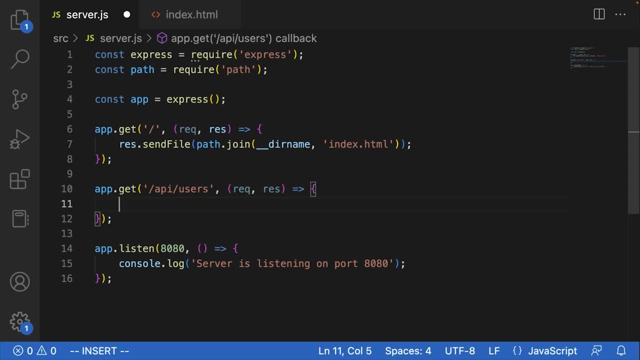 an array of JavaScript objects, each of which represents some sort of user data. So what that's going to look like is we're going to say const users equals, and then our first user will just have an ID of one, two, three, four, five, six, seven, eight, nine, ten, eleven, twelve, thirteen. 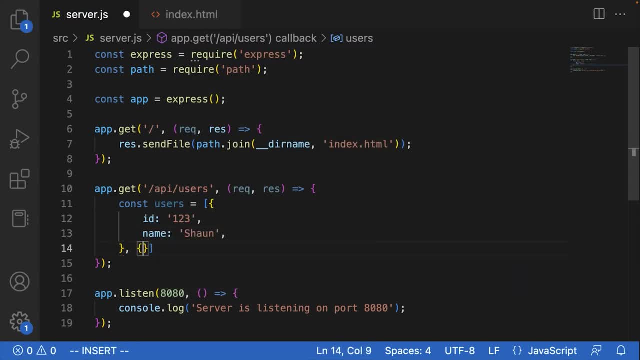 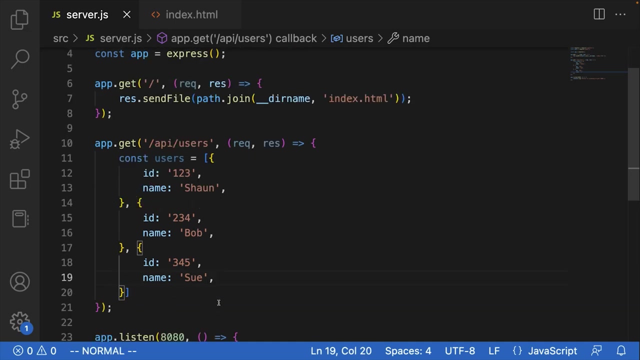 and the name: we'll do Sean, And then the next user will say ID two, three, four, name. we'll do Bob, and then ID three, four, five, name: Sue. Okay, So this is obviously very simplified user data, but the same process would apply regardless of how complex our data is. So now that we have 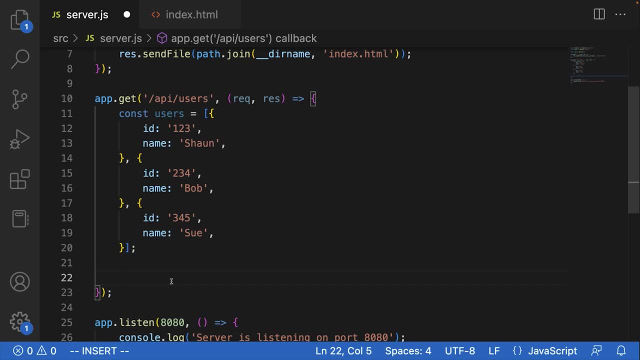 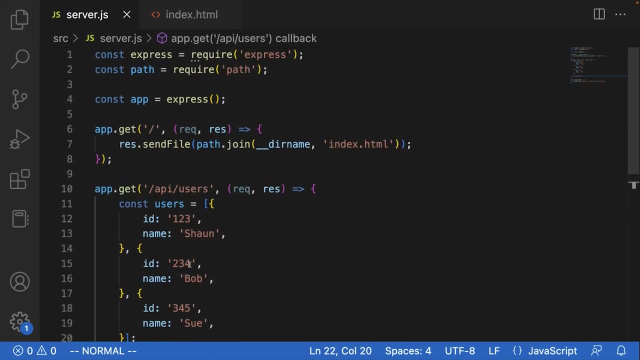 those users. we're just going to send them back to the client side by saying response dot userjs. And then we're going to send them back to the client side by saying response dot JSON users. Okay, So now that we have these two endpoints, what we're going to do is head over to 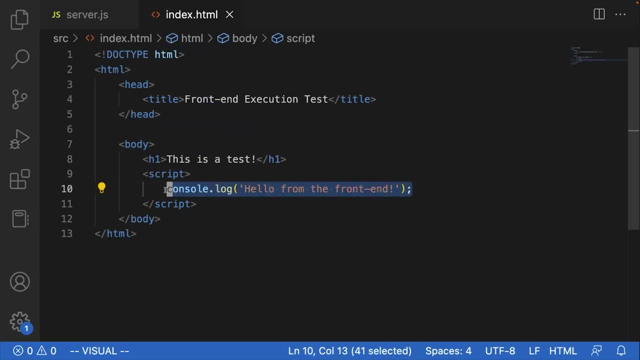 the front end, And instead of just logging something out to the console directly, we're going to have our front end code make a request to the backend. Now you might wonder how this is done programmatically. right, We were able to make a manual request just by entering in a URL to the. 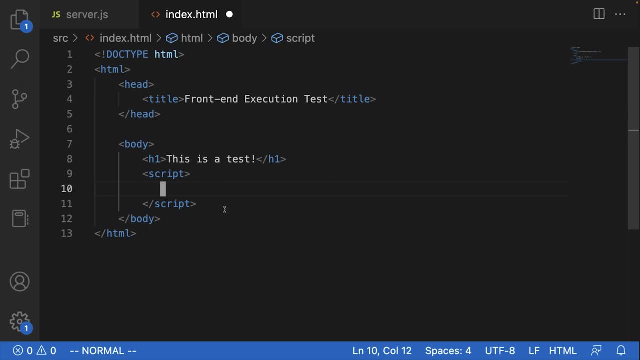 browser and hitting enter, But when we want our code to do it, there's a specific function that we're going to use most of the time on the front end, And that function is called fetch right, And, in fact, if you want to learn more about this, just look up the fetch API. This is a default. 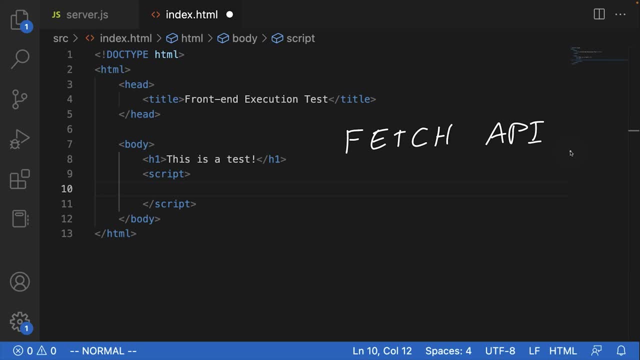 API that we can use in front end code that we can use to do things like send network requests. Okay, So using the fetch API is a pretty straightforward process, Really. all that we have to do in most cases is say: fetch right, And this is automatically included. right It's. 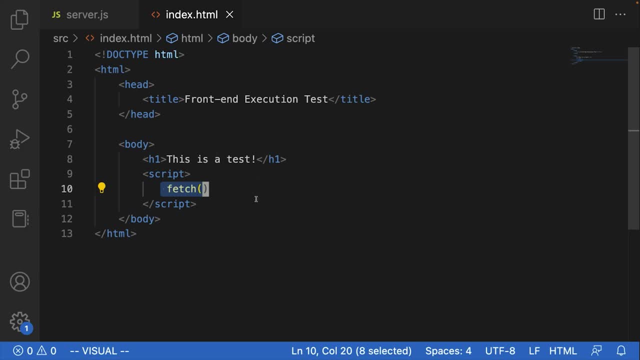 automatically available in our JavaScript code here We don't need to import it or anything, And the fetch function can take a number of arguments, but the simplest way to do it is just to pass the URL that we want to send this request to as the first argument. So what this? 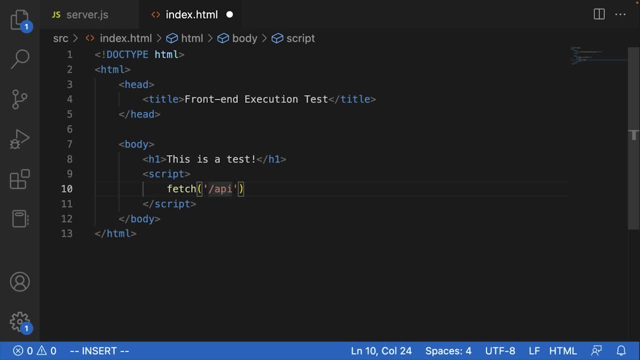 is going to look like is we're going to say slash API, slash users. Okay, And notice that we didn't need to include the full localhost 8080 thing, because this indexhtml file is coming from localhost 8080. So that's just where the browser is automatically going to send these requests that we make with no 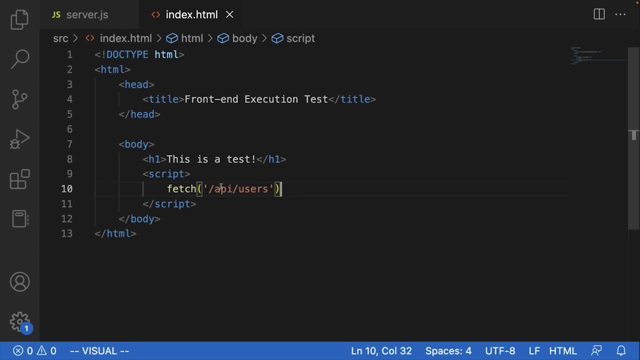 domain name. Okay, So saying fetch slash API, slash users is going to send a request to the back end and the default request type, of course, is a get request. So if we just want to send a get request to do something like load data, which is the case here, all we need to do is say fetch with the URL. 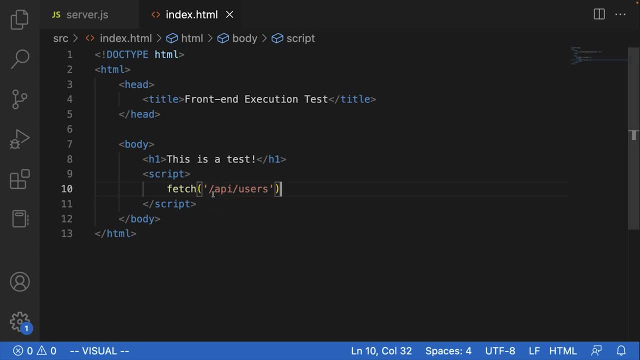 We don't need to specify any kind of options or any other arguments. We'll see how to do that later on, So the next thing that we're going to need to do is deal with the results of this fetch call. Now, obviously, network requests such as this: 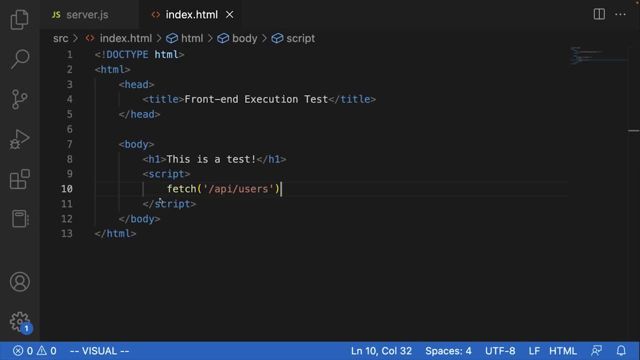 one are asynchronous, right, They take a long time. So in order to avoid blocking the main thread, the fetch API is going to use promises. Now, what this means is we can get the result of calling fetch by just adding dot then onto the end of it. 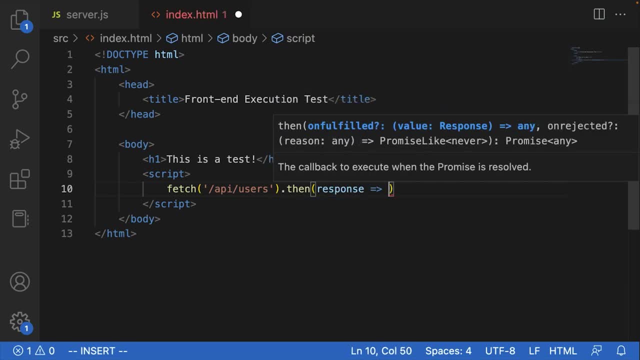 So we're going to pass a callback function to this That is going to take the response as an argument and inside this callback function, Now we can do whatever we want with that response. All right, Now one thing to know about this response that we get back from the fetch API is that, in order, 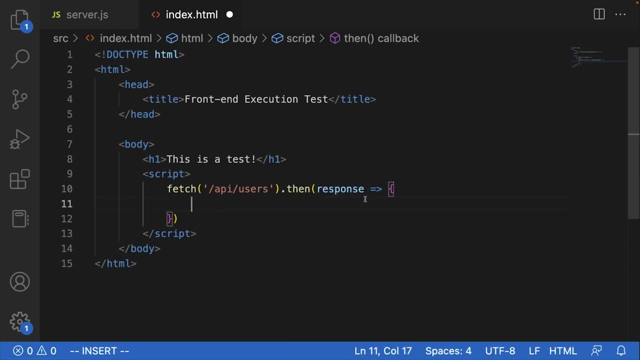 to get the data it contains. we actually need to call another function and return that from this dot. then callback, right. So we're going to say response dot JSON and this will give us a JavaScript object or array, whatever the service sent back to us that we can work with. So all that we need 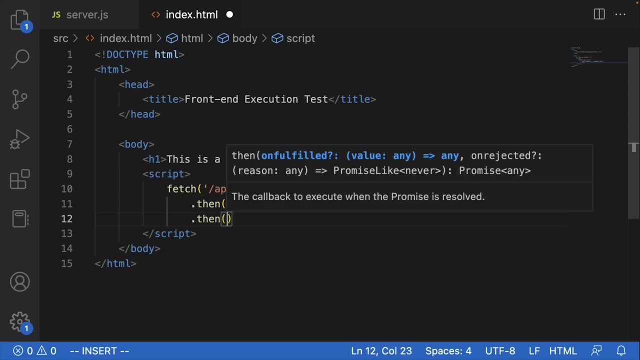 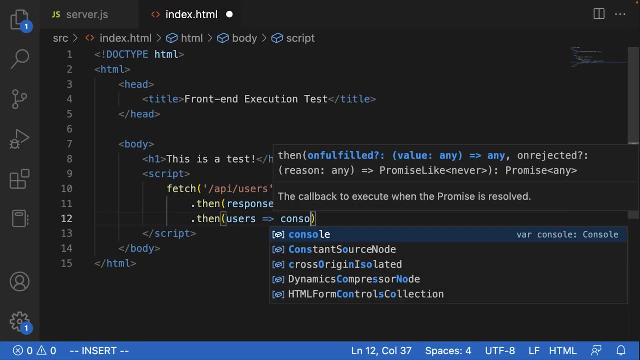 to do now is add another dot then onto the end of this and that will be the actual data right, That's going to be our users that the server sent back. So now what we can do is just say console, dot, log, and we're going to print those users out to the console here. You could also display them. 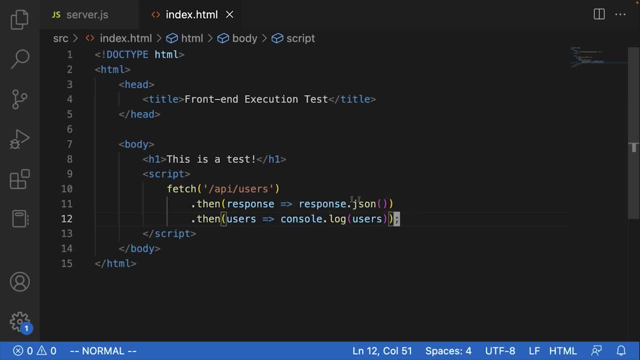 in an alert if you wanted to, but using console dot log is usually the way that's recommended to you know, debug and take a look at the results of JavaScript code. So that's really all that we need to do Again. 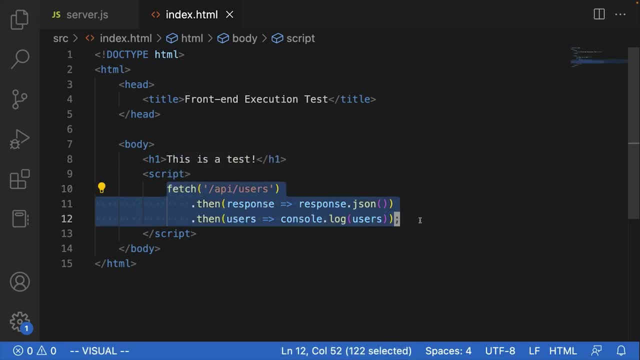 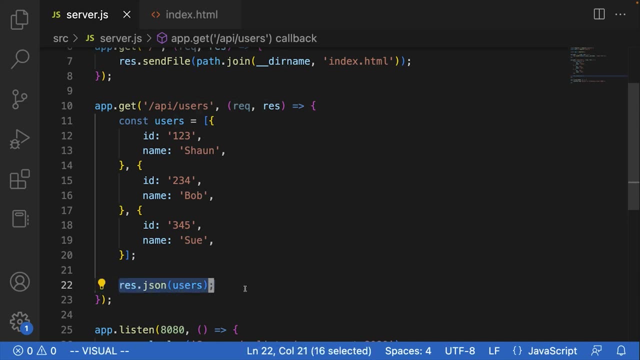 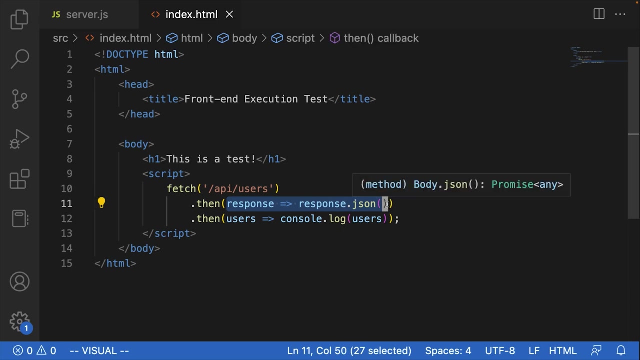 what this is going to do is, when the browser runs this, it's going to send a request to the endpoint that we defined on our server, And this is going to send back the array of user data which will then be passed to this callback function. We're going to convert that into an actual JavaScript. 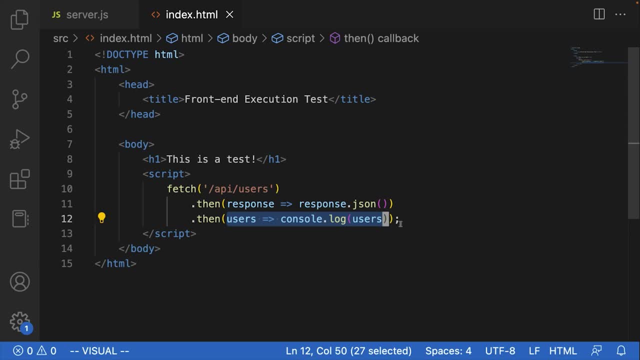 object and we can use that final result inside this callback here. For now, all we're doing is logging that out, So let's run this thing and see if it works. What we're going to do is, first of all, you'll want to make sure that your server has restarted successfully. It looks like mine has. 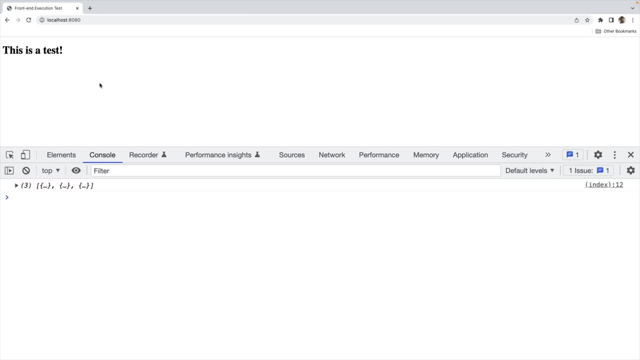 And now, if we go back to the browser and hit refresh, sure enough, what we'll see is that inside the console here, after our code has completed, it's logged out the user data to the console and we see that we have all of our user data right here. So in other words,